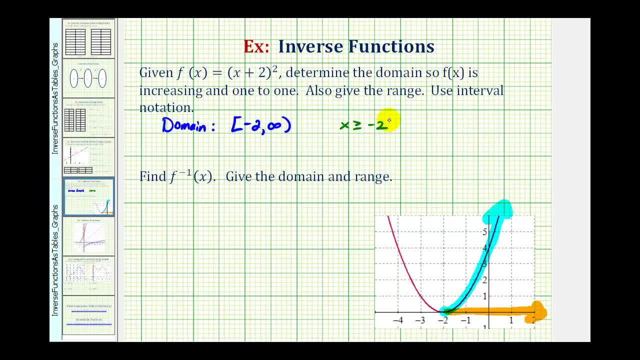 as x is greater than or equal to negative two. Now let's consider the range. The range is a set of all possible y values or outputs of this function on the restricted domain. Well, if we project this graph onto the y axis, notice how the smallest y value would be zero. 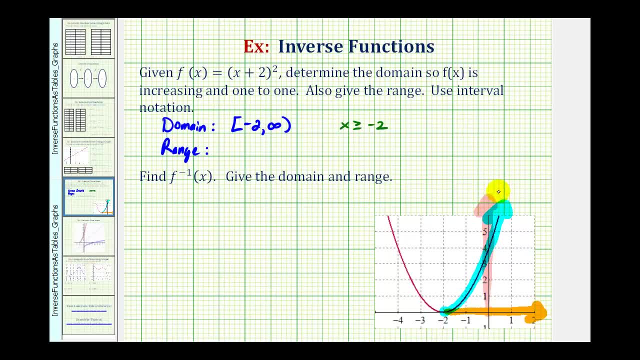 and from there it increases upward toward positive infinity. So the range would be the interval from zero to infinity, closed on zero, meaning it includes zero. or we could say y is greater than or equal to zero. With this restriction, the function f is now one to one. 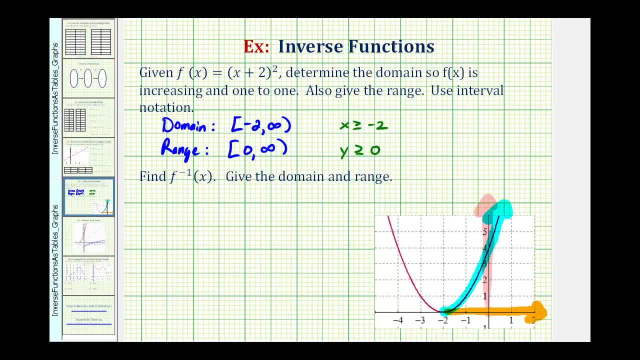 so we can find f- inverse of x. To do this, let's first write the original function replacing f of x with y, So we'd have y equals the quantity x plus two squared. and then, to find the inverse, we interchange the x and y variables and then solve for y. 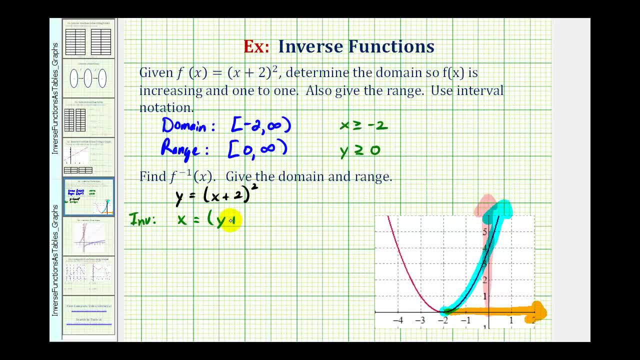 So we have: x equals the quantity y plus two squared. and now we'll solve this for y, The first step. we'll take the square root of both sides of this equation. So we'd have the square root of x equals the square root of the quantity y plus two squared. 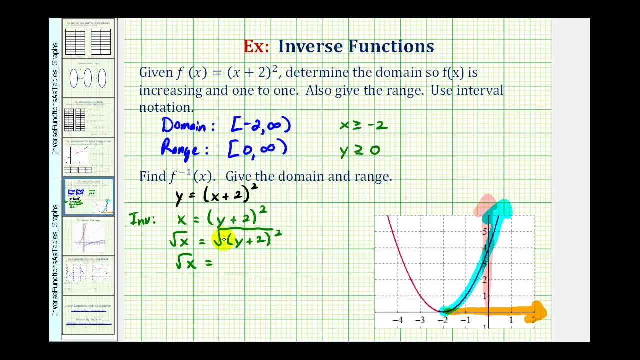 So we have the square root of x equals. normally this would be the absolute value of y plus two, but because of the restrictions here we don't have to worry about that. This would just be y plus two. Last step: we'll subtract two on both sides. 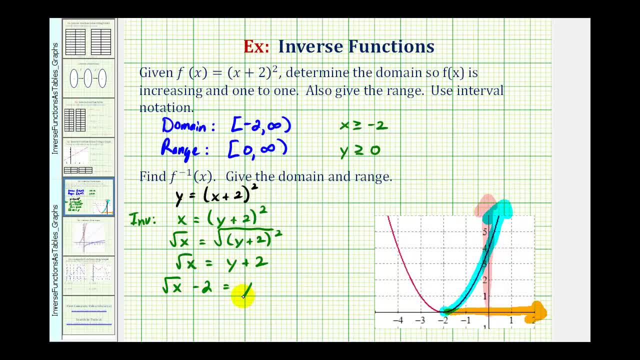 We have: the square root of x minus two equals y. This is our inverse function: solve for y. So we'll go ahead and replace y with f- inverse of x. f inverse of x is equal to the square root of x minus two. 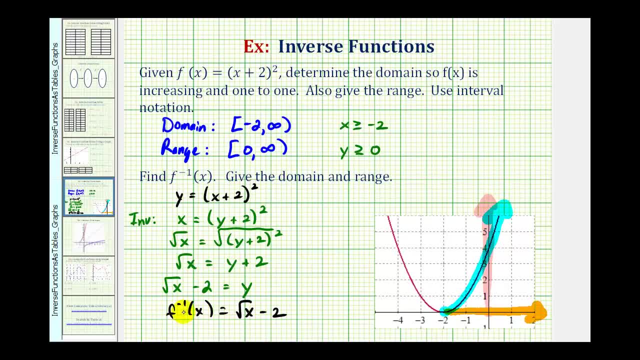 And we're also asked to give the domain and range. so let's go ahead and do that, Because this is the inverse of function f. the domain of f is going to be the range of f inverse and the range of f will be the domain of f inverse. 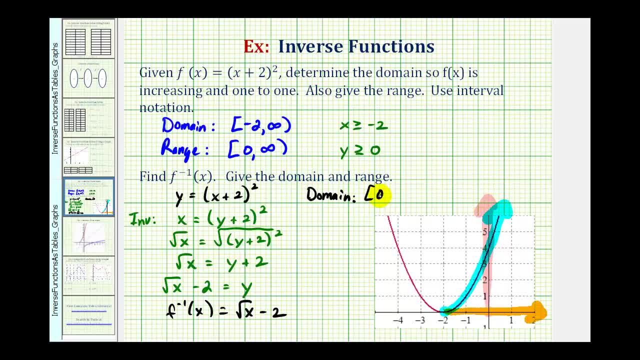 So the domain will be from zero to infinity, closed on zero, and the range will be the interval from negative two to infinity. Let's go ahead and finish by verifying this graphically. We know that if we graph function f on the restricted domain,